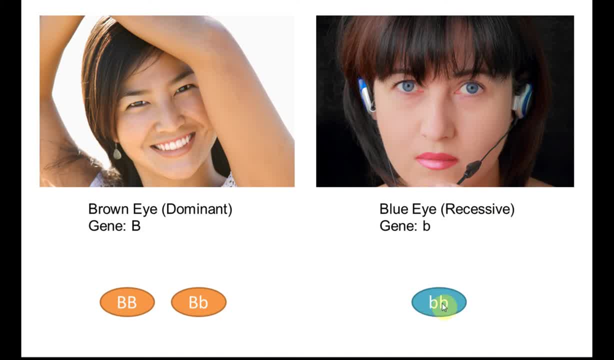 In the organisms. Okay, for example, both of the genes are blue eye and therefore these ladies has blue eye. Okay, so this is a difference between the dominant genes and the recessive genes. The dominant gene is a very powerful genes which will be shown in the organisms. Okay, and 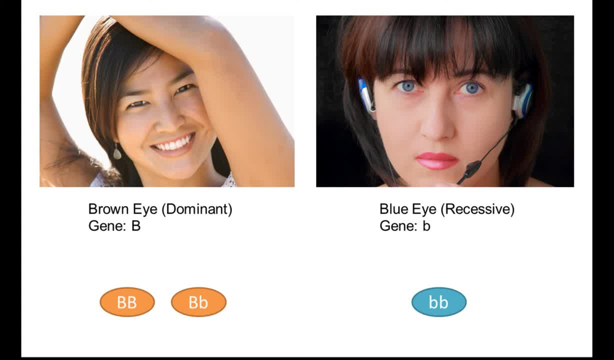 recessive most of the times. Okay, it will be just stored inside the chromosome. Okay, unless both of the genes are recessive, then only it will be shown in the organisms. okay, so this is the meanings of dominant genes and recessive gene. okay, so here is a list of the dominance and recessive. 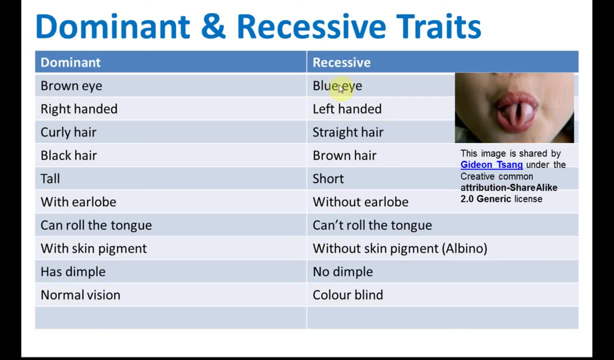 genes. brown eye is dominant and blue eye is recessive. right-handed is dominant and left-handed is recessive. curly hair is dominant and straight hair is recessive. black hair is dominant, brown hair is recessive. tall is dominant, short is recessive. the ear with earlobes is dominant and without. 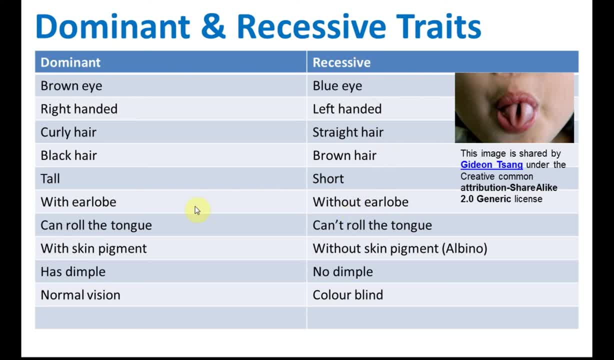 earlobes is recessive. i will show you the pictures after this. okay, can roll the tongue. okay, this is what does it mean? okay can roll the tongue is dominant. can roll the tongue is recessive with skin pigments. dark skin is dominant. without skin pigments- for example albinos. we will discuss that later. it's recessive and has dimples. 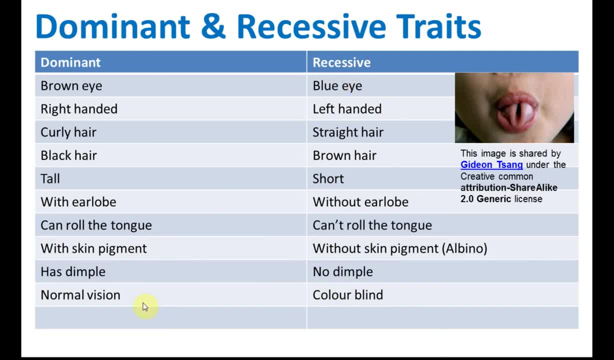 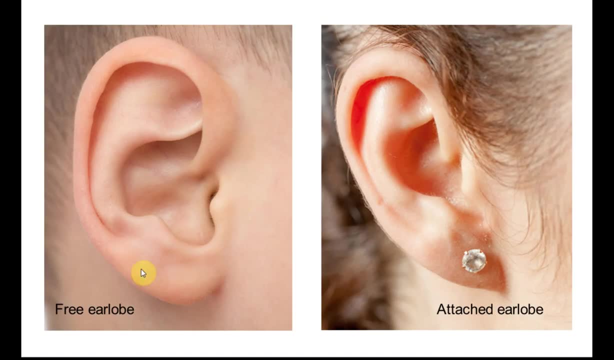 is dominant and no dimples is recessive. normal, нашей readership is dominant and colorblind is recessive. okay, and you need to remember this. which one is dominant and which one is not dominant, recessive, you need to remember, okay. so this is what does it mean by free ear? 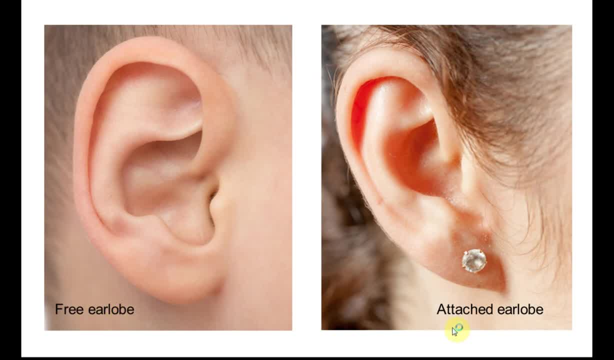 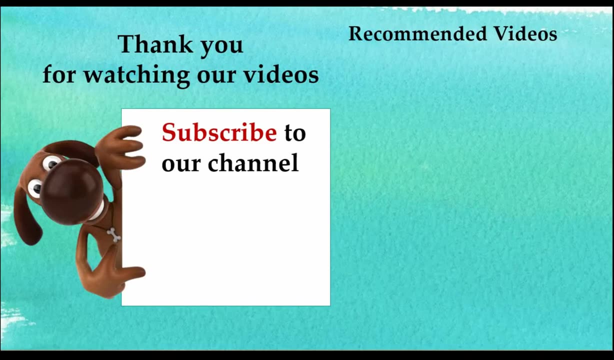 looped. okay, this is free ear looped and this is attached ear loop. we can see that this ear loop is attached to the face and this one, the ear loops, is not attached. so it's free ear loops and attached ear loop you.